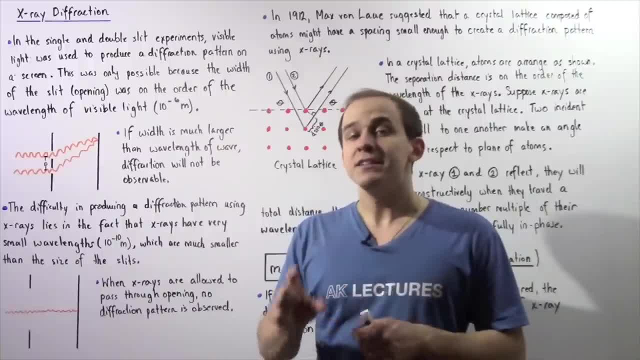 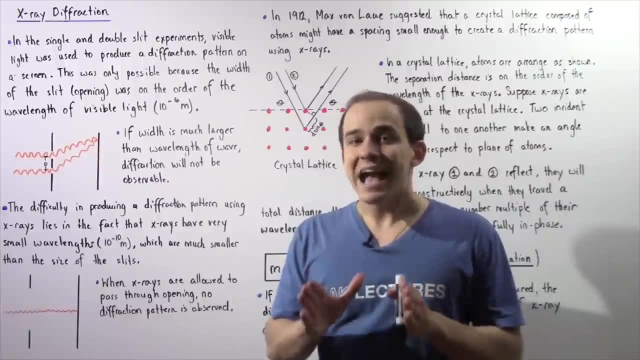 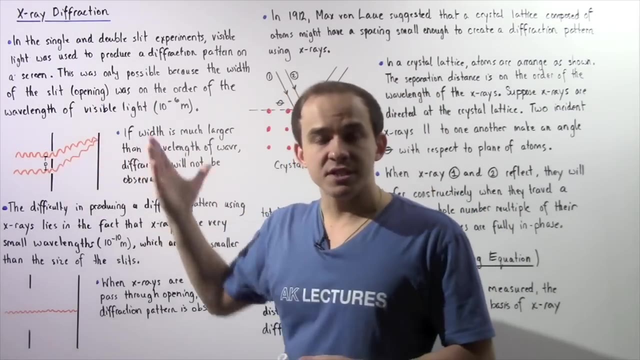 radiation is much smaller than the size of the openings, then no diffraction pattern is actually observed. Now that's exactly what happened when scientists tried to essentially point the x-rays at these double slits. No diffraction took place. That's because the size of the wavelength 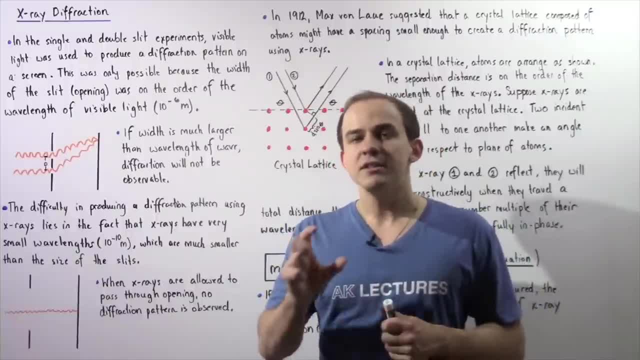 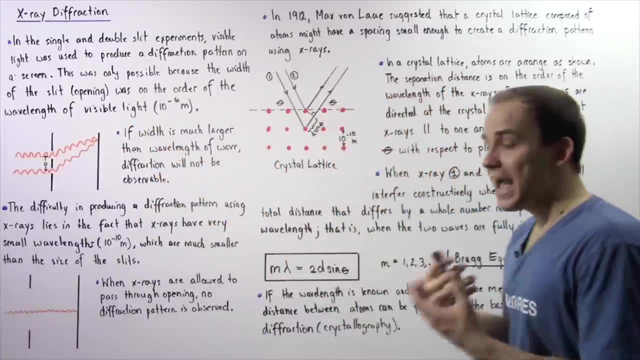 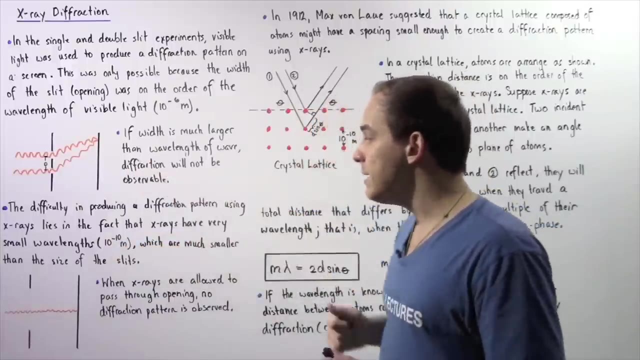 of x-rays is much, much smaller than the size of these openings. So the difficulty in producing a diffraction pattern using x-rays lies in the fact that x-rays have a very small wavelength, about 10 to negative 10 meters, which is much smaller than the size of these. 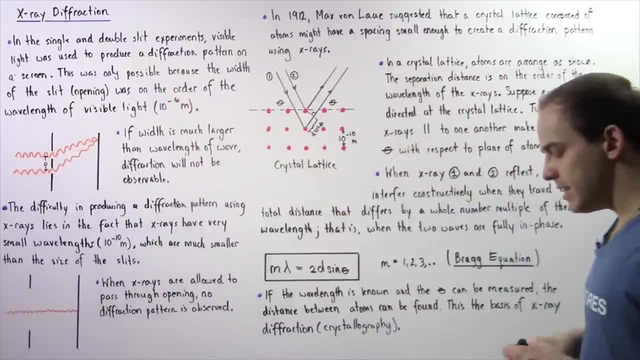 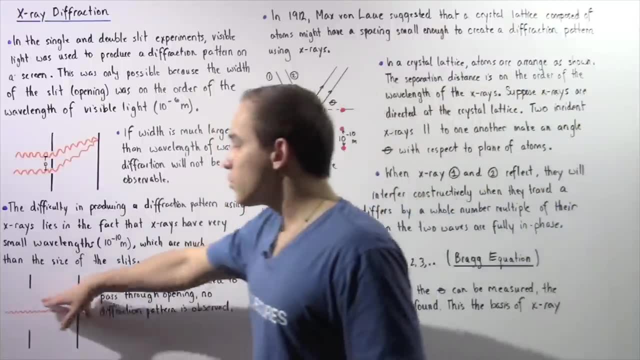 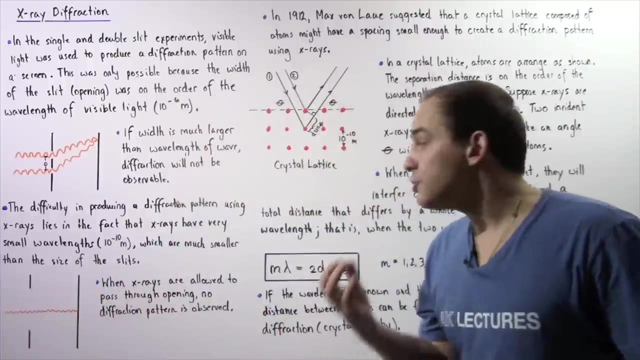 slits, which is about 10 to negative 6 meters. So basically, when scientists took those and they allowed those x-rays to pass through the openings, these openings were so large compared to the wavelength of those x-rays that no diffraction actually took place. 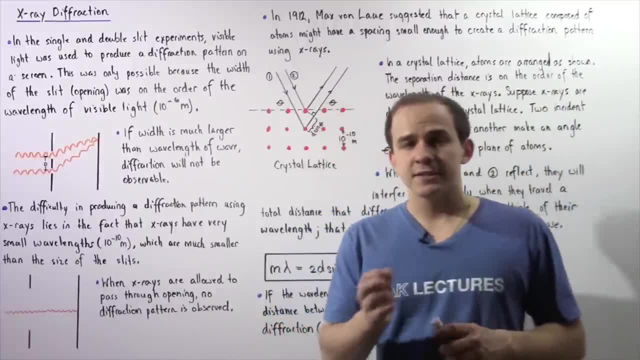 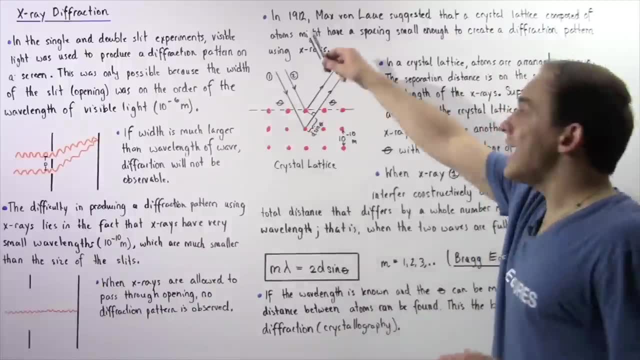 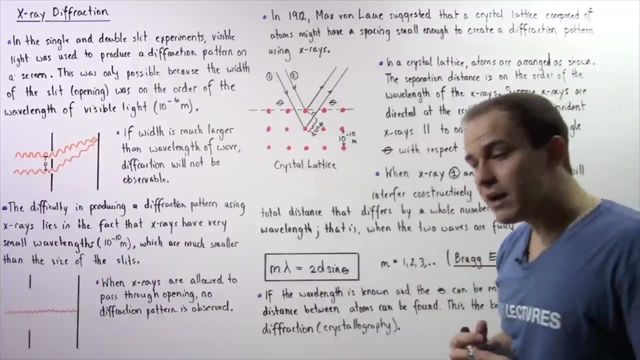 Now, in the year 1912, a German physicist by the name of Max von Laue came up with a clever solution to this problem. So in 1912, Max von Laue suggested that a crystal lattice composed of atoms might just have a spacing between the atoms that is small enough. 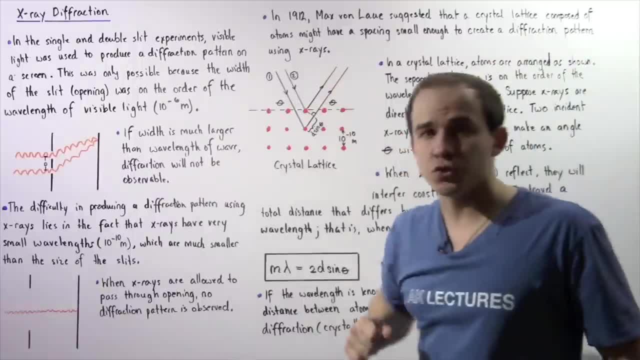 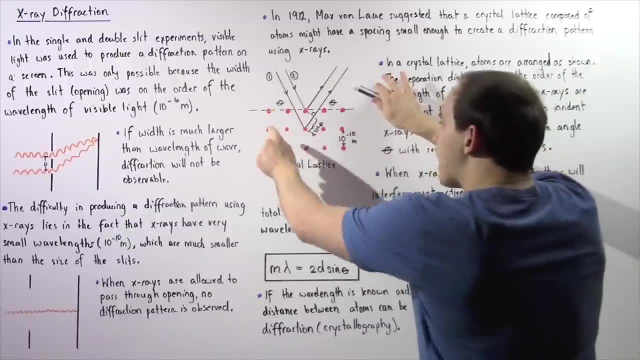 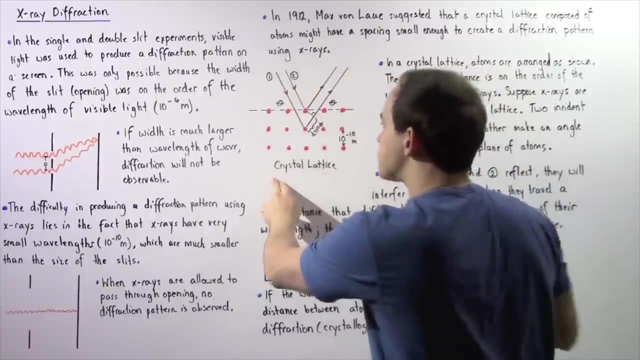 to actually create a diffraction pattern using x-rays. So to see exactly what we mean, let's look at the following diagram. So these red atoms are our atoms that form the following crystal lattice that looks like this: So let's suppose we have x-rays which are coming as shown in the following diagram. 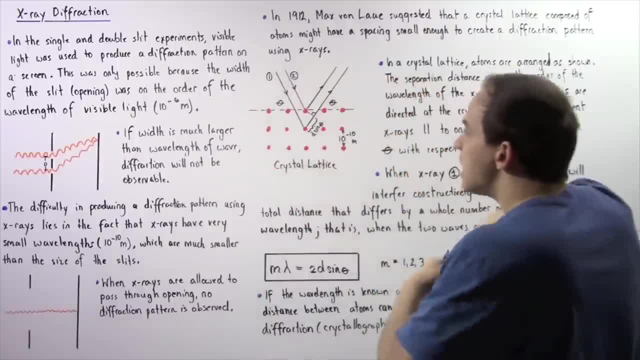 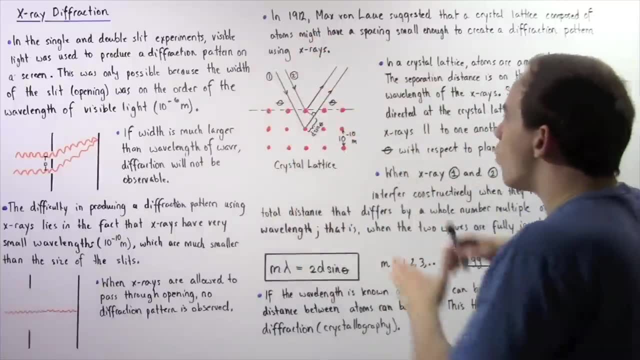 So we have x-ray 1 and x-ray 2.. Now, because they're coming from very far away, we're assuming they're parallel with respect to one another. Now, when they hit the following plane of the crystal lattice, shown by the following dashed line, 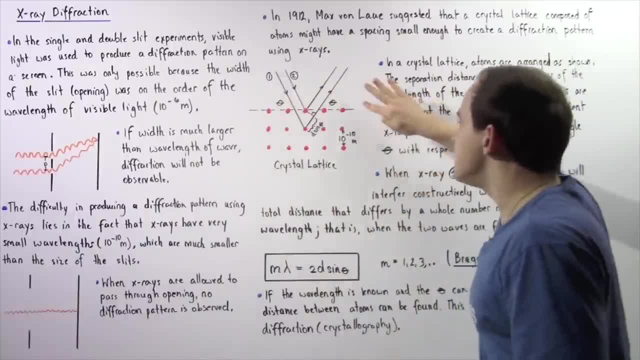 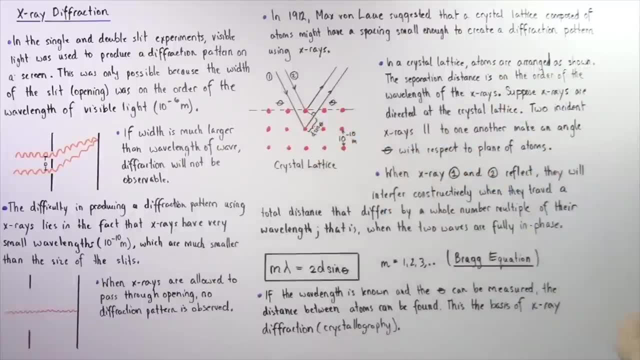 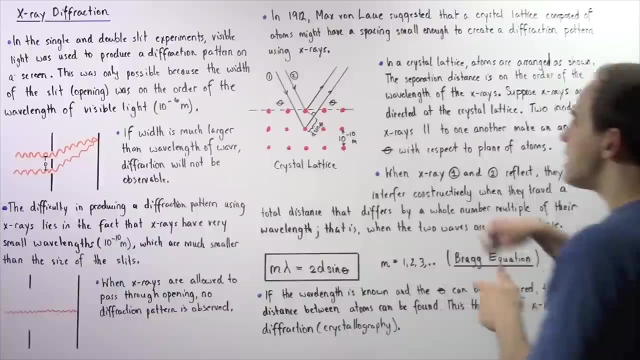 they make an angle, theta, with respect to this plane. So once again, in a crystal lattice, atoms are arranged as shown in this diagram. Now, the separation distance is on the order of the wavelength of the x-rays. In fact, the distance between our two atoms is 10 to negative 10 meters. 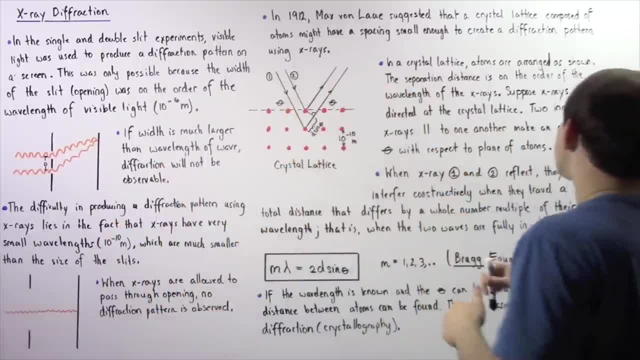 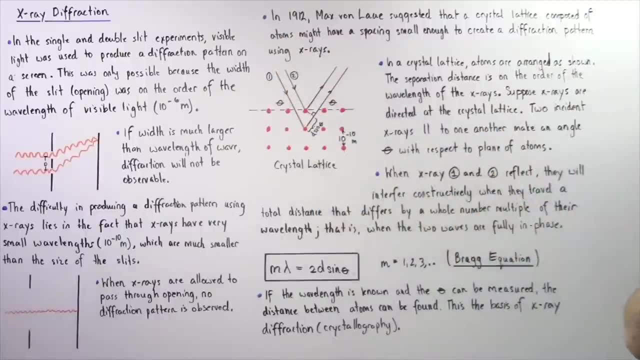 which is about the same as the wavelength of our x-rays. Now, two incident x-rays, as shown, are parallel to one another and make an angle theta with respect. So the plane of the atoms. Now, when x-ray 1 and x-ray 2 reflect, 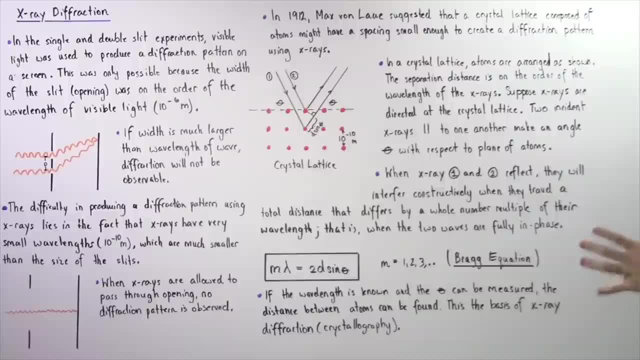 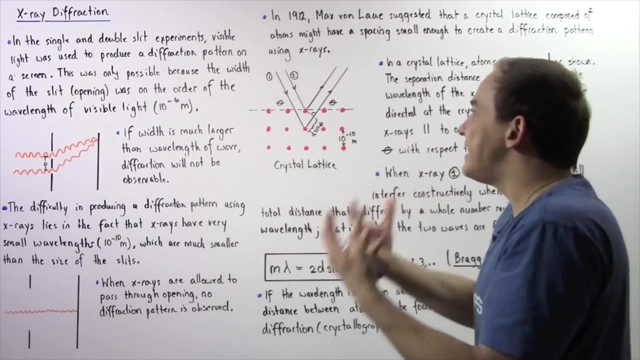 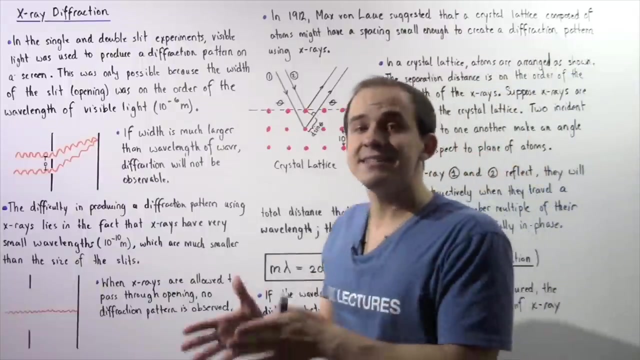 they will interfere constructively with one another when they travel a total distance that differs by a whole number multiple of their wavelength, That is, these two waves once they actually reflect. they will interfere constructively only if the distance they travel, the difference in that distance, is a whole number multiple of their wavelength. 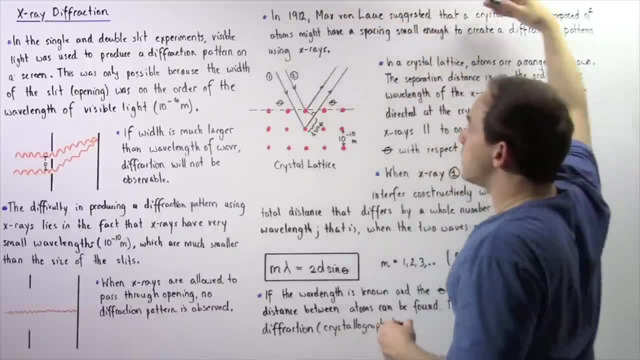 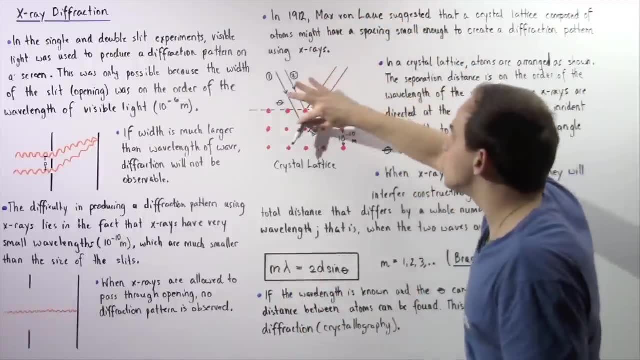 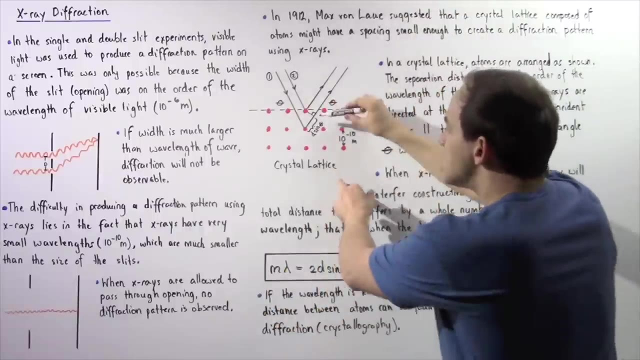 So basically notice- let's suppose we have the screen somewhere here- This upper wave, wave number 2, will travel less than this lower wave, And that lower wave will travel a distance of d sine theta less. So basically, if this is equal to a whole number multiple, 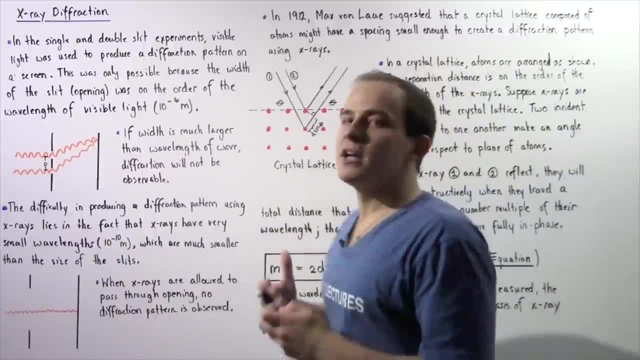 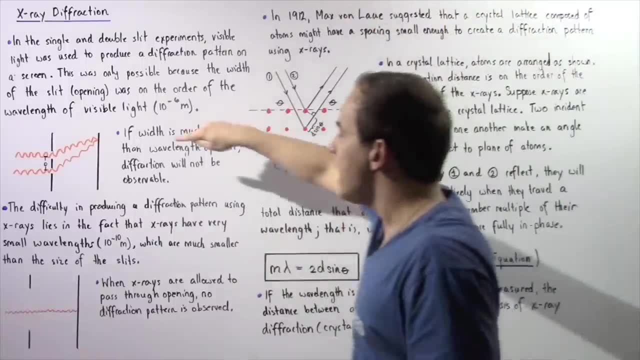 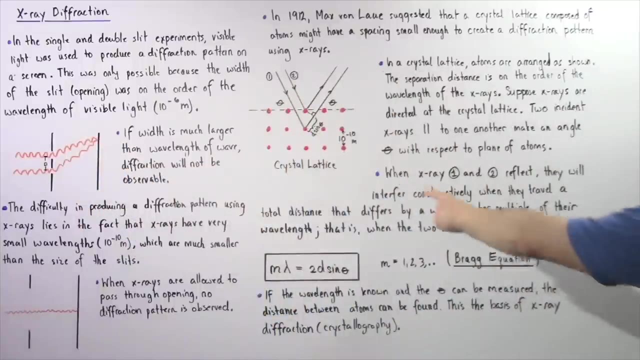 then that basically means they will interfere constructively and they will form bright fringes on some viewing screen, in the same way that bright fringes were formed in the following double slit experiment. So once again, when x-ray 1 and x-ray 2 reflect, 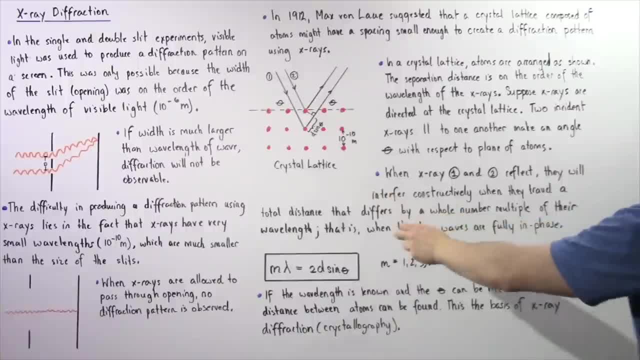 they will interfere constructively when they travel a total distance that differs by a whole number, multiple of their wavelength. That is when the two waves are fully interlinked. That is when the two waves are fully interlinked And the equation that gives us this relationship. 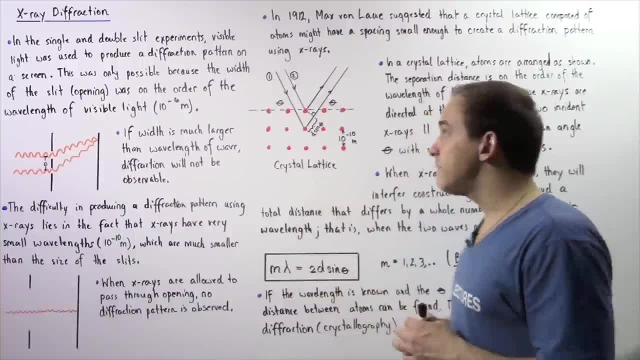 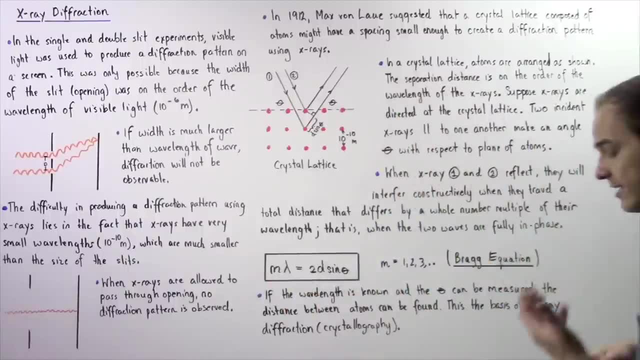 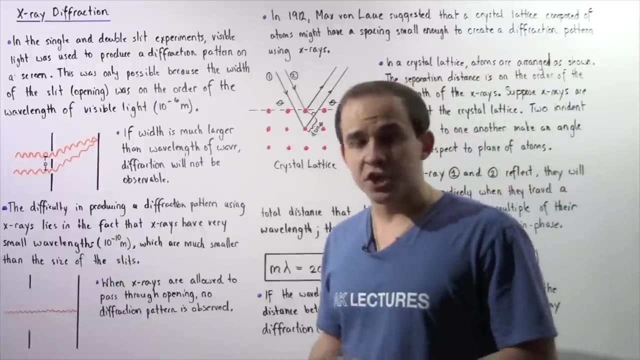 that gives us the location where they will interfere constructively is given by this formula, which is known as Bragg equation, after the English physicist who essentially derived it. Now, m is simply a positive integer. It could be 1,, 2,, 3,, 4, and so on.